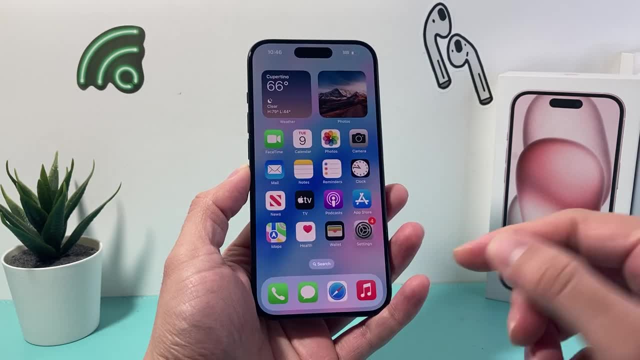 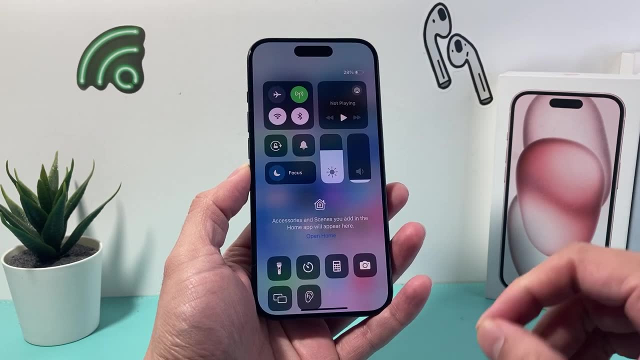 So let's get started. So the very first thing is: first thing, you want to ensure that your phone has at least 20% or more charge, And you can pull down the control menu here, see the charge percentage. And the reason why that is is because once the phone goes under 20%, 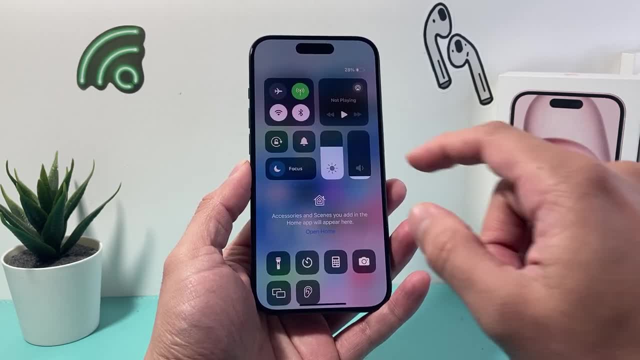 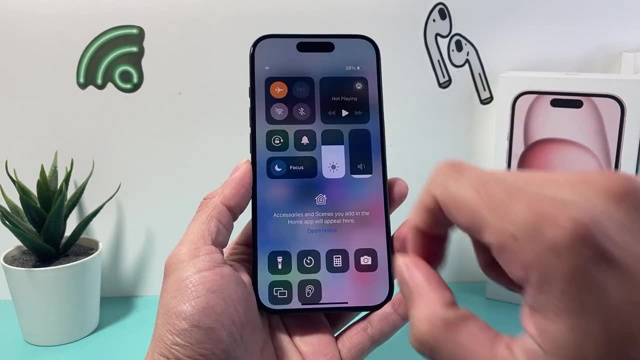 certain things start becoming limited functionality, like Wi-Fi and Bluetooth, to save battery. So make sure your phone is charged up Now. after that, the next troubleshooting step is we're going to put our phone on airplane mode briefly and then turn it back off. 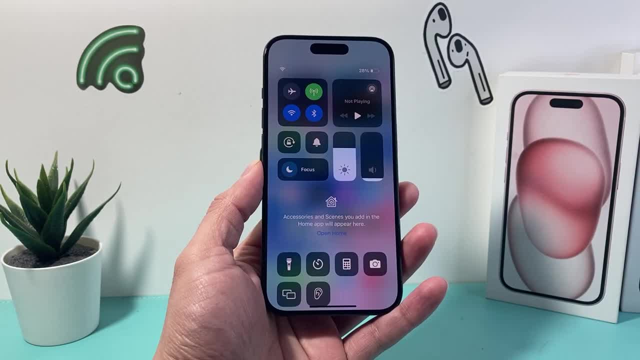 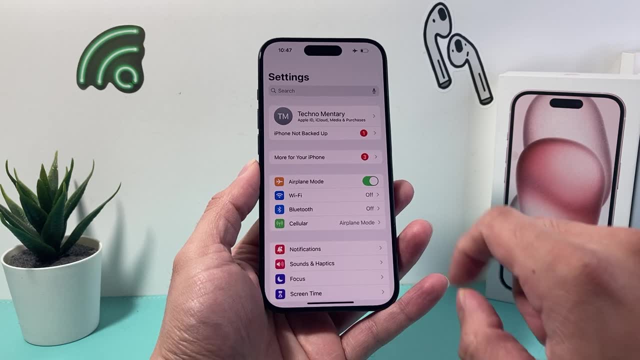 And it does a quick network refresh. As you can see here, my Wi-Fi and the Bluetooth is working. After I do that, you can also do this from the setting by going into your settings and then turn on Bluetooth here, right, And then turn it off. just like that It does a quick network refresh. 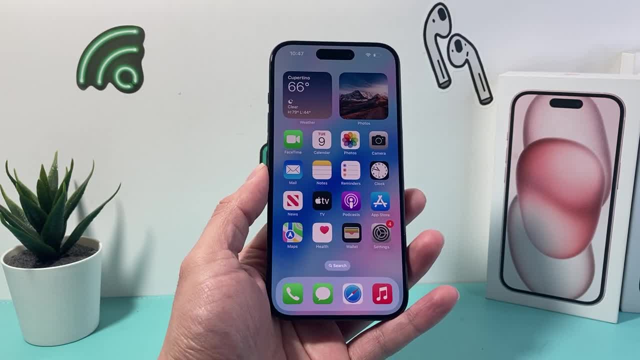 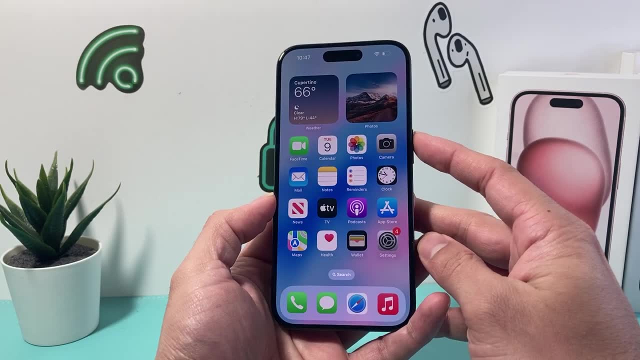 Now, if that didn't help, the next thing you want to do is a forced restart on your iPhone. In order to do that, you're going to press and release the volume up, press and release the volume down, one after another, and then hold the side button until the screen goes completely black. 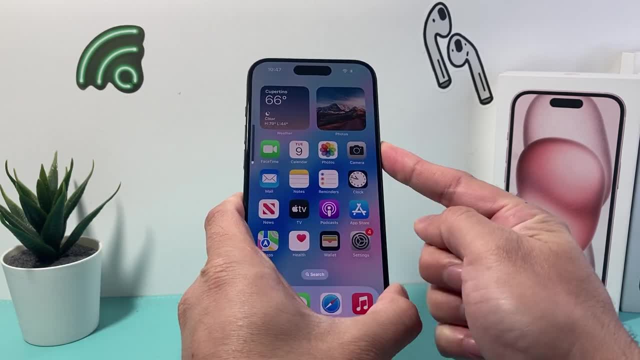 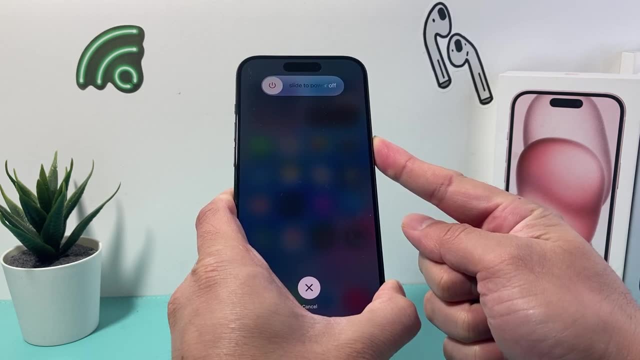 So I'm going to do volume up, volume down, and then I hold on to that side button. While I'm pressing and holding, there's going to be a pop-up that comes up to slide to power off. But you do not need to do that because that will be a normal turn off. 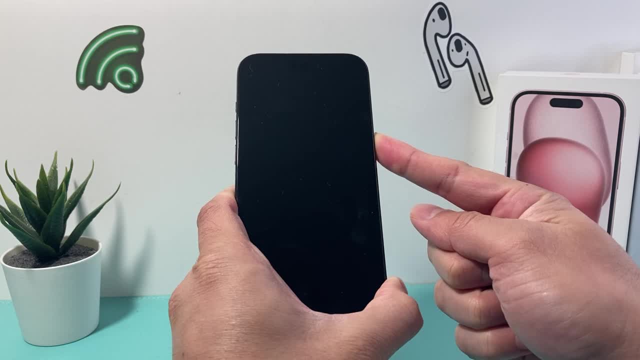 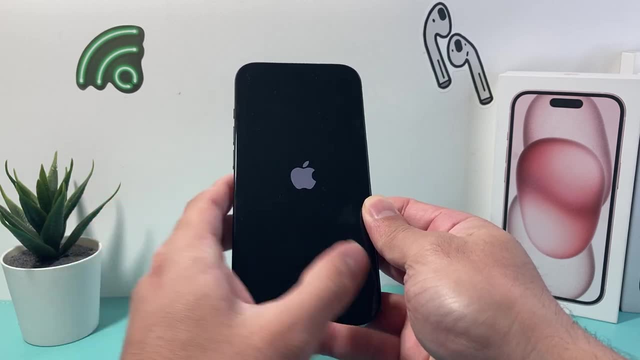 We want to make sure it's forcing itself to shut down, And once you see the Apple logo, you'll let go of that side button. Again, you want to do it quickly: Press and release the volume up, press and release the volume down, one after another, before holding on to that side button. 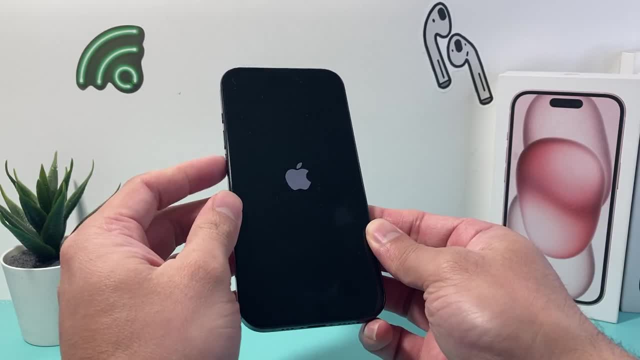 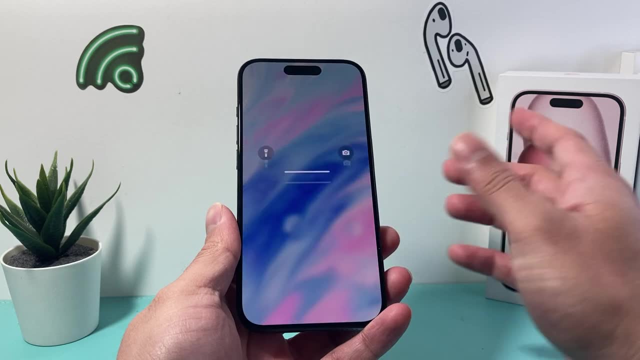 Now, this might take you a couple of times to get it right, So if it doesn't work the first time, keep on trying. And this method just basically shuts down the software and reloads the code. It's safe. It will not delete any of your personal data. 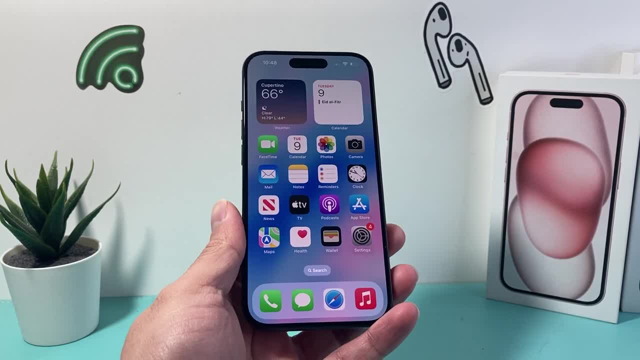 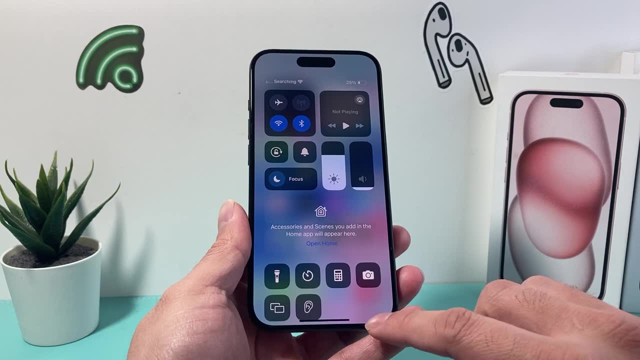 All of your photos, videos, apps will still be on your phone, So you don't have to worry about any of that. Now, if it's still not working, where you're getting your Bluetooth or Wi-Fi still being not working or grayed out? 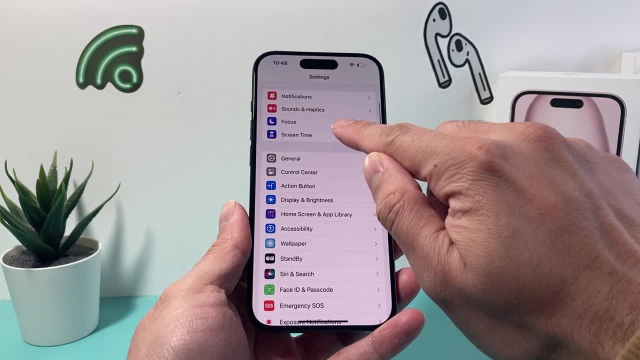 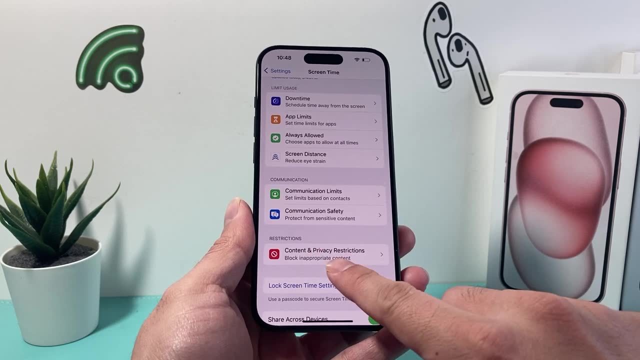 the next thing to troubleshoot is going to your setting of your iPhone. Click on screen time and you might have a screen time passcode that you might need to enter. But once you do that, go down to restriction, where it says content and privacy. 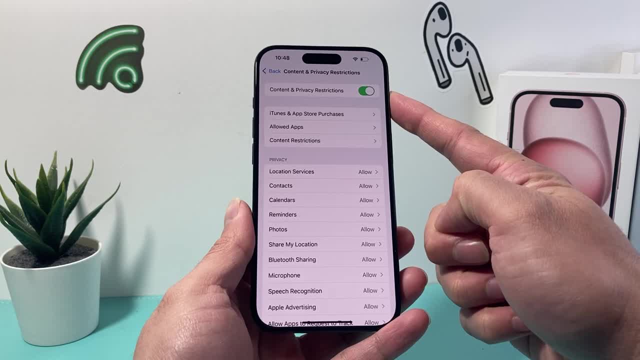 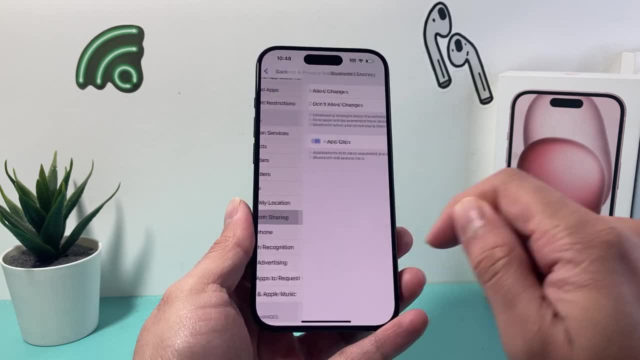 You want to click on that Now. if you have content and privacy restriction turned on, you want to follow this. If you don't have it on, you can skip this part, But if you do have it on, you're going to go down here where it says Bluetooth sharing. 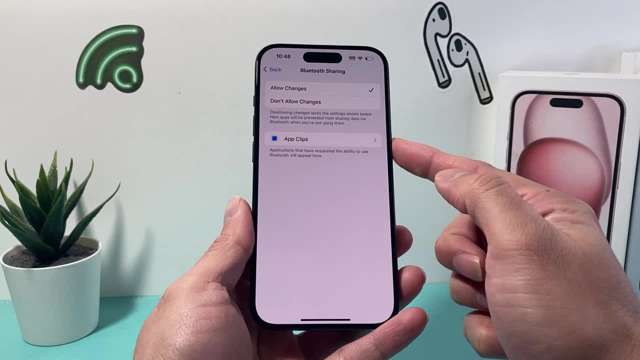 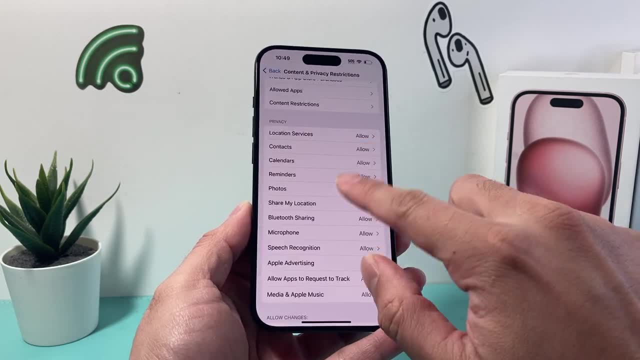 Make sure that it's selected to allow changes And, under app clips, if you have apps that need Bluetooth, make sure they're turned on if you have apps listed here. So you want to ensure that Now, after you have done that. 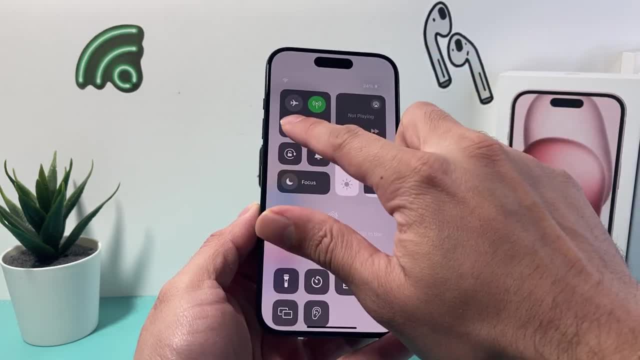 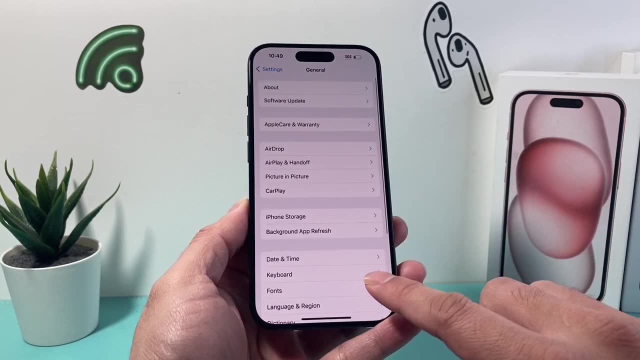 and if it's still not working, you might still see that your Bluetooth on the Wi-Fi is still grayed out. The next thing to do is go into your setting of your iPhone, go to general, And this time you're going to want to go scroll down. 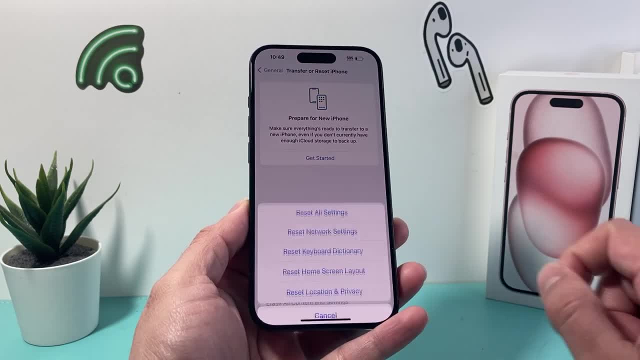 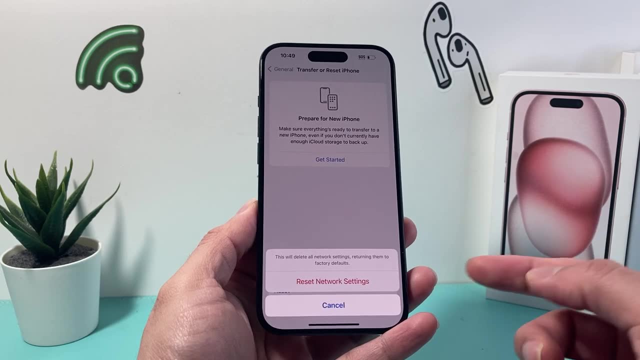 which is transfer reset iPhone. You're going to click on that and then click on the first option to reset, which will give you the menu to reset network setting. You'll click on network resetting. Basically it'll reset all the settings, like saved Wi-Fi. 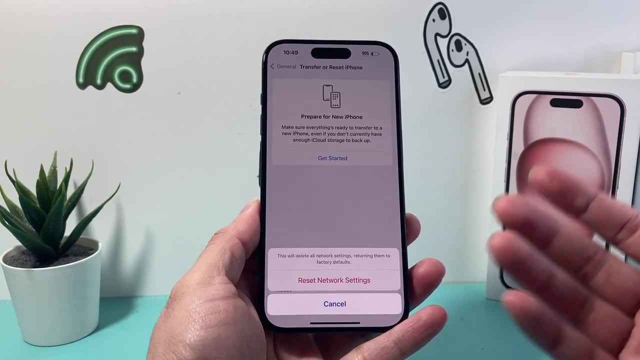 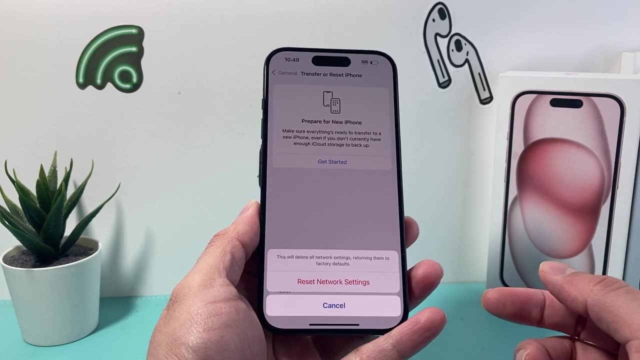 any Bluetooth connected devices, but that's simply fine because you want to do that if you're having issues connecting with Bluetooth or Wi-Fi And you click on that. it will take about a minute or two to do And this method again will not delete any of your personal data. 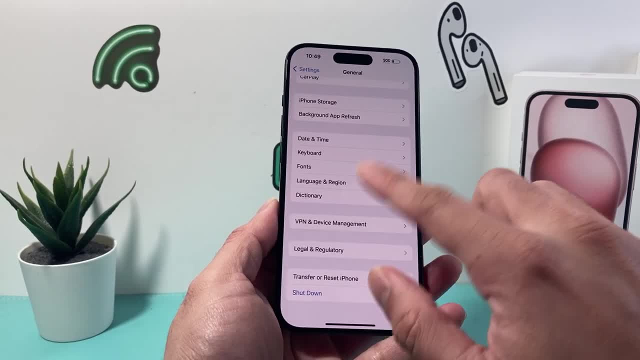 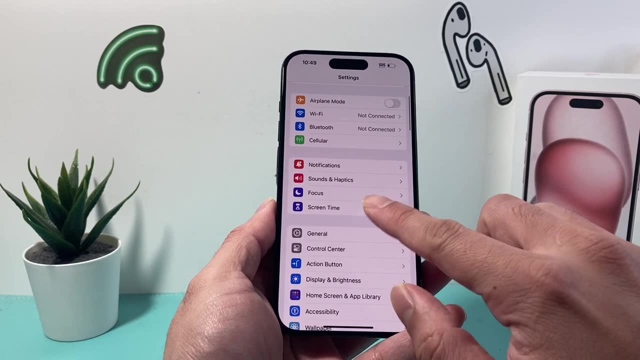 So all of your photos, videos, apps will be safe. After doing that, hopefully it's working Now. if it's still not working where your Bluetooth and Wi-Fi are still grayed out, the next thing to do again in the settings. 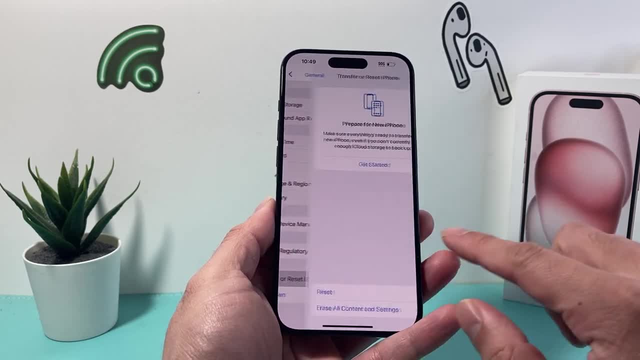 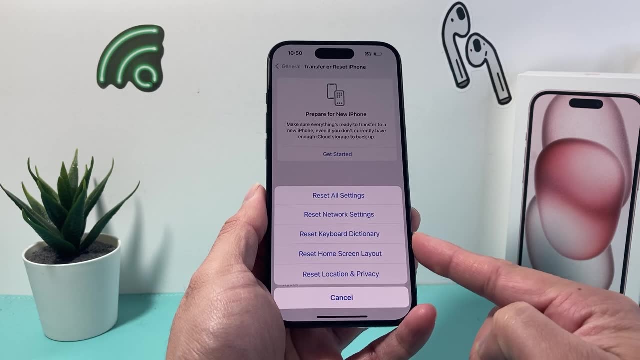 same thing again. we're going to go to general, scroll down to transfer, reset, iPhone, click on reset And this time we're going to do all a setting reset which basically will do a reset of all the settings, like network related settings. 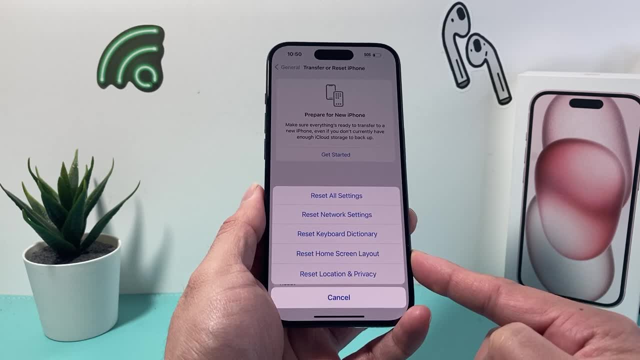 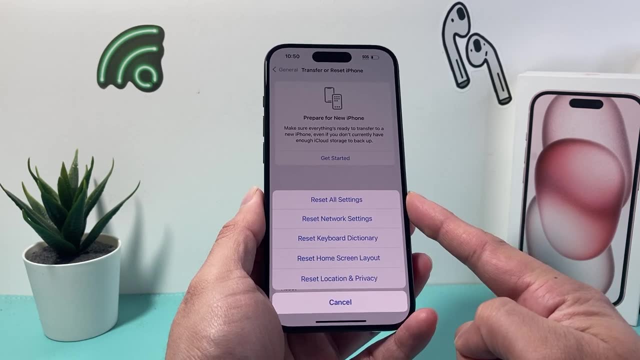 your keyboard dictionary setting home screen layout settings. If you had a customized home screen layout, it will just get reset any location and privacy settings themselves. So all this is going to do is reset all the settings, but it's kind of important to do that. 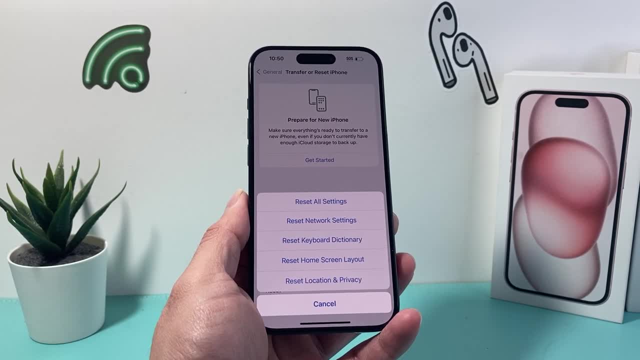 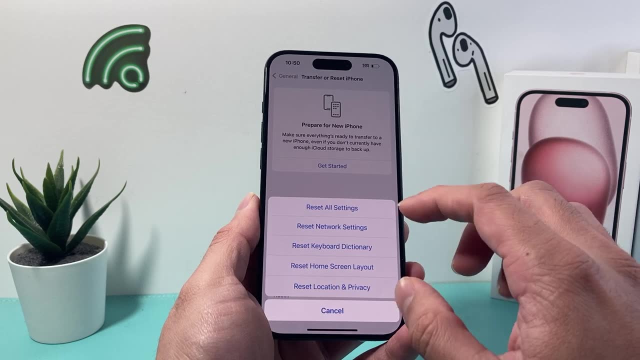 if you just simply can't get Wi-Fi or Bluetooth to work or they're still grayed out, And this will generally take about a minute or two to do Again. it will not delete any of your personal data like photos, videos, apps. anything will not get deleted. 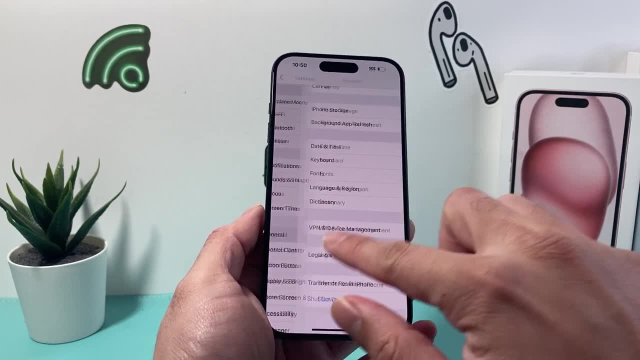 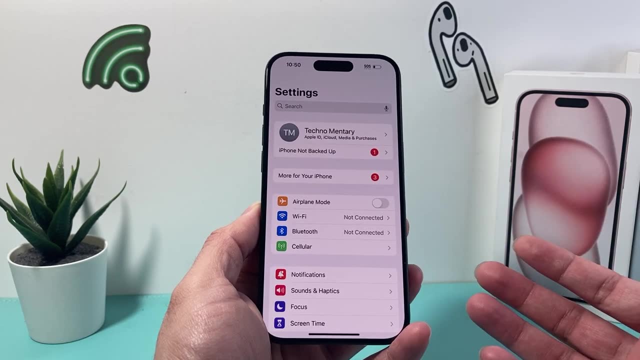 just like it says here, but something you'll need to do in order to fix it Now. if that didn't work for you, the next thing to do is see if you can update your phone Now. to update your phone, you can try using cellular data. 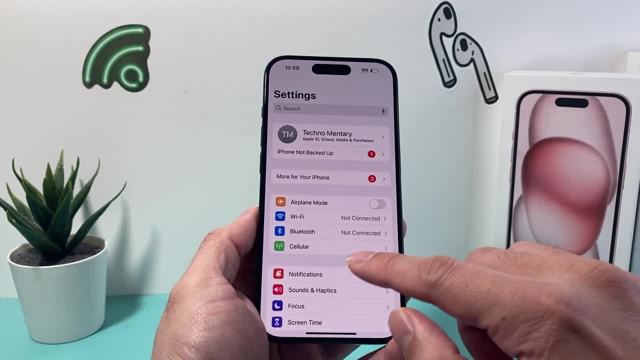 if you have cellular data, but if you don't have cellular data, you'll need to go. If you have cellular data, you'll go here general software update and you'll update here Now if you get unable to check for update.